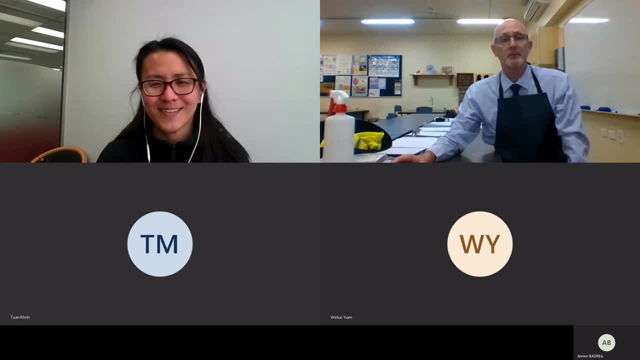 demonstration I'm going to do. Hello, Eamonn, how are you? Hi? Hi, You're being recorded, so if you're going to speak and I'll be asking you questions, you need to speak very loudly and clearly, please. Okay, is that good? 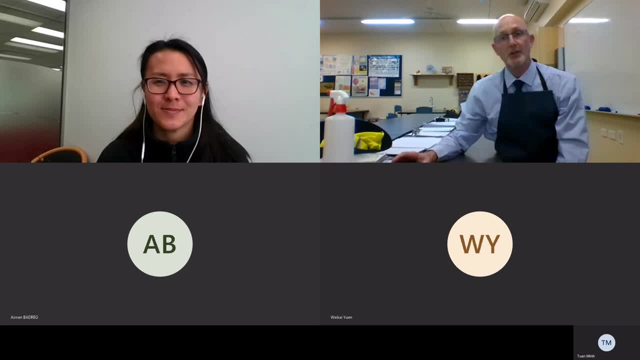 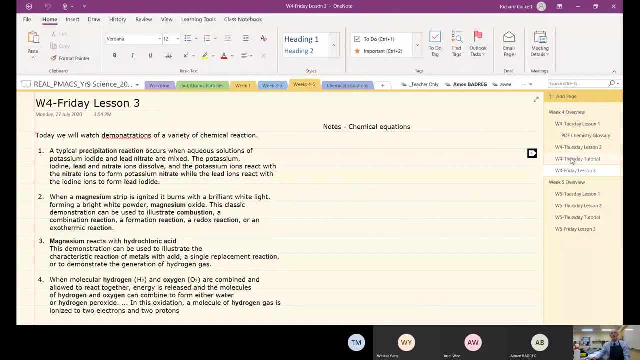 Good, excellent. So I'm going to do some demonstrations now. Okay, the first one. Now let me just share my screen again and show you what you should be looking at. Okay, this is our class. one note, So there's Thursday's lesson. 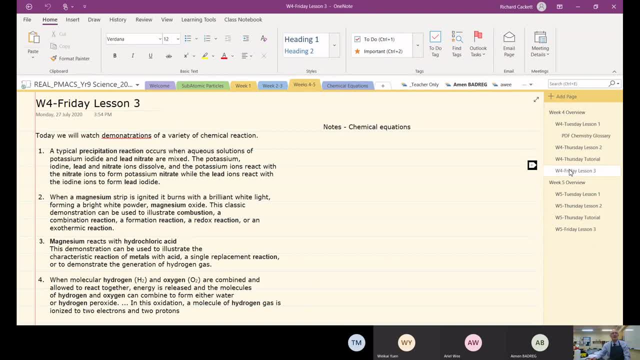 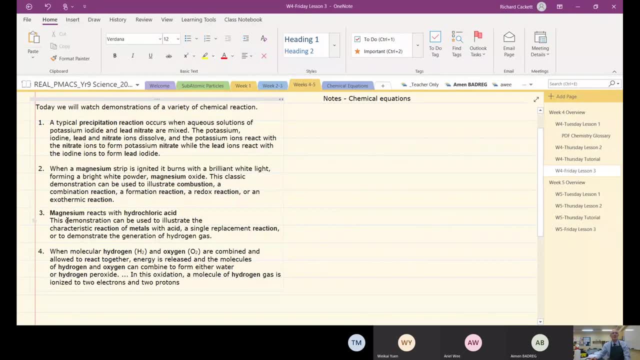 And today's lesson. So let me quickly correct that spelling mistake Done. So there are four experiments I want to demonstrate to you. So that's what I'm going to be doing today. You've got copies of these and you're going to be making notes. 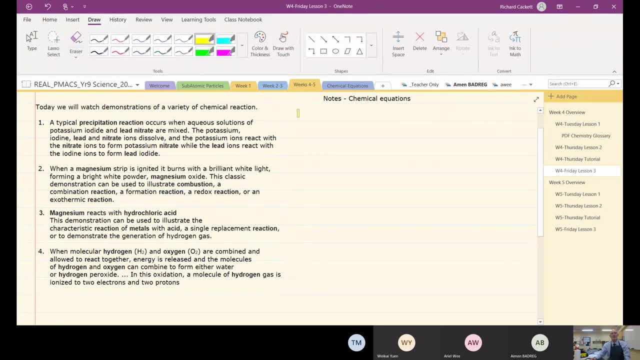 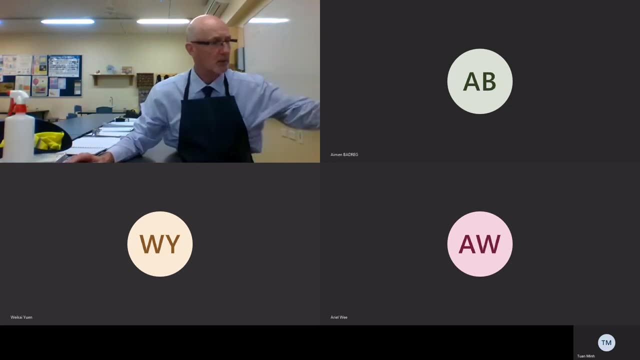 Okay, you're going to be making notes in this area. Get around here. Okay, this is where you're going to put your notes. So back to live cam, Here we go. So the first experiment I have got. So the first experiment I have got. 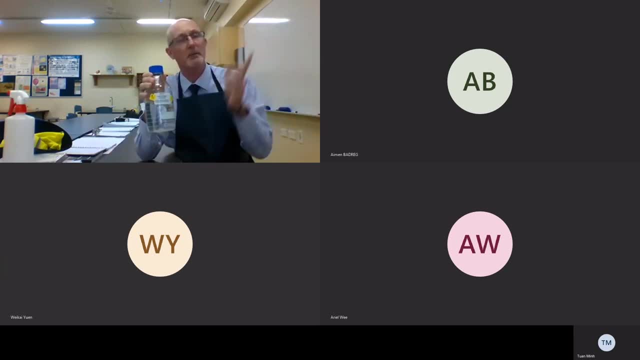 lead nitrate- If I'm looking sideways, it means I'm looking at a big screen. Lead nitrate, A clear liquid. I've got potassium iodide and again I'll be writing down the formulas for these and we'll balance them shortly. So two clear liquids. 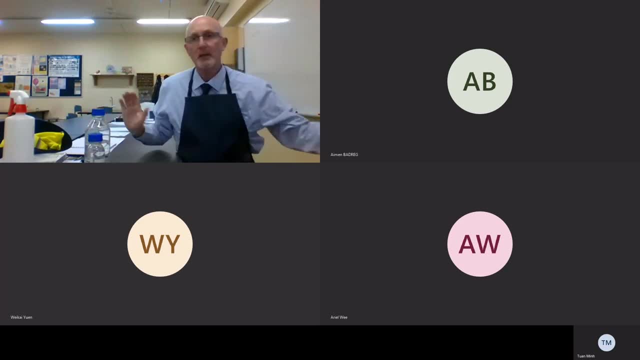 We're looking at chemical reactions. So I have a beaker and I'm going to carefully. I'm not going to measure, I'm just going to pour a truckload in, because it's a demonstration and I want you to see it. So, Hello Willem, how are you? 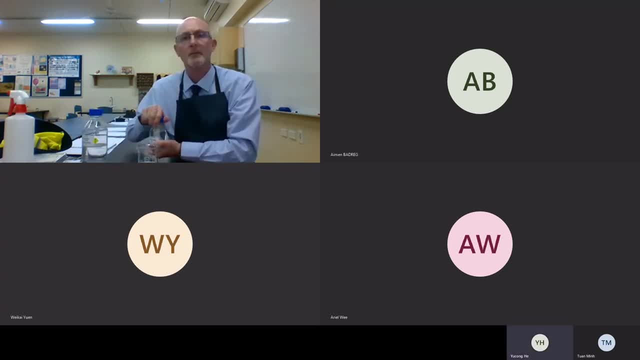 Hi, Hi, sir, Good afternoon. Just a quick warning: You're being recorded, We are all being recorded. So if you're going to speak, speak loudly, please, and clearly. Okay, so demonstration: Lead nitrate Clear. Now we've got potassium iodide. Now this is what we call a precipitation. 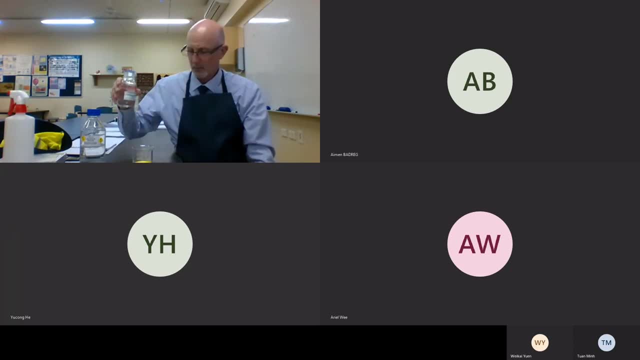 So if I add this, Okay, we get a yellow substance forming. So, two clear liquids, Two clear liquids. Add them together, We get a yellow solution. Now, if I wait a while- but I won't be able to- then that yellow substance will actually sediment, it will drop and it'll be a thick layer at the 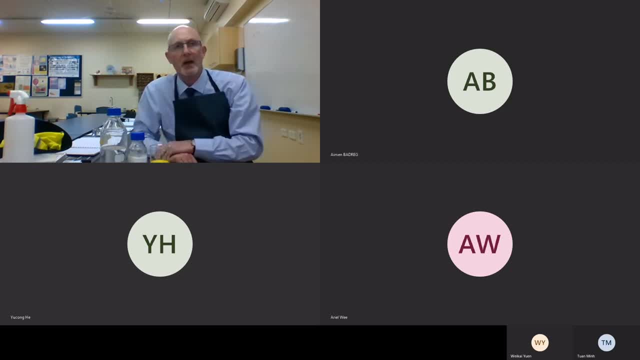 bottom. so what we have produced is a precipitate. so we have two aqueous liquid solutions and when we combine them, there's a chemical reaction and we get a solid, insoluble product being made. so I'm using a few words now that we're getting used to. so we've got reactants and we have products. so 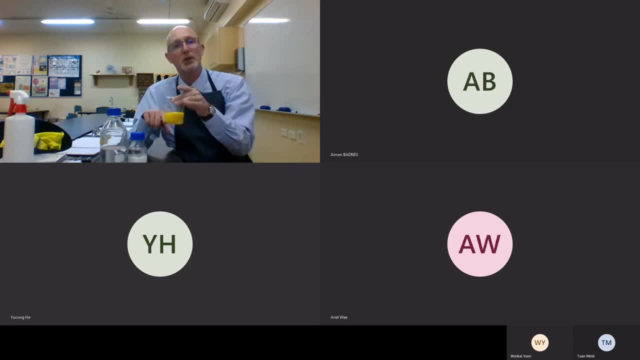 there are two products in here. one will be a liquid, one will be a soluble, insoluble, solid. so that's the first reaction. any questions? no, okay, okay, we'll look at the chemical equations that in a minute. just put this over here, right? our next reaction is things oxidation. so we're looking at. 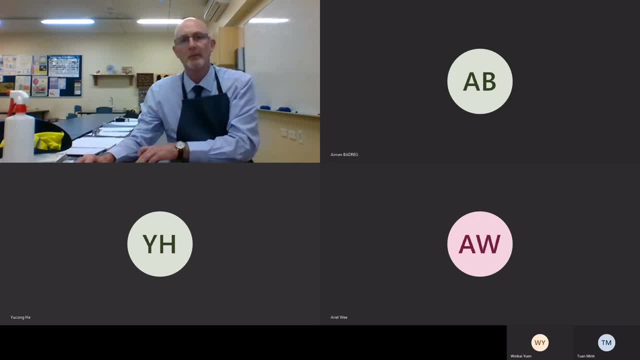 magnesium ribbon. so magnesium ribbon is looks something like that: magnesium. if you look at the periodic table- okay, it's in those seconds column. it has an atomic number 12.. okay, it's a metal. so it's shiny, malleable. we can bend it, we can stretch it out and make it into wire like we have here that's called ductile. okay, it will. 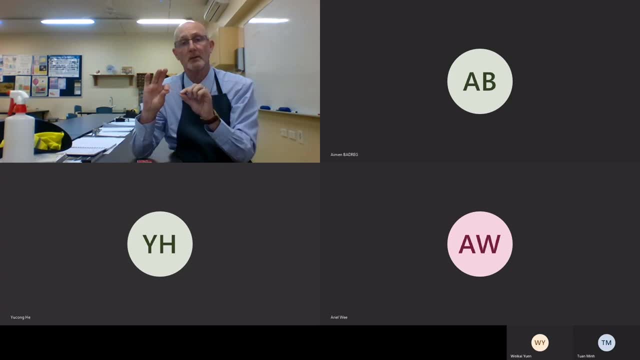 conduct heat and it will conduct electricity as well. so there are some of the properties of metals. now, how much oxygen is in the air we breathe? what percentage? 10, 20, 30, 40, 100 percent? someone take a stand 41. so, Ricky, you're getting 41 percent, okay, amen, would you like 41, 21.. yes, no, that's better. yeah, so it's around 18.8%. 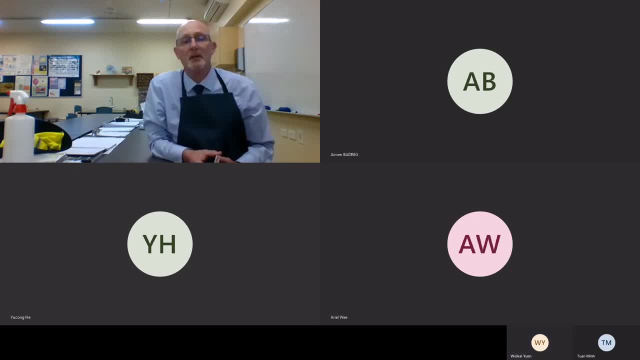 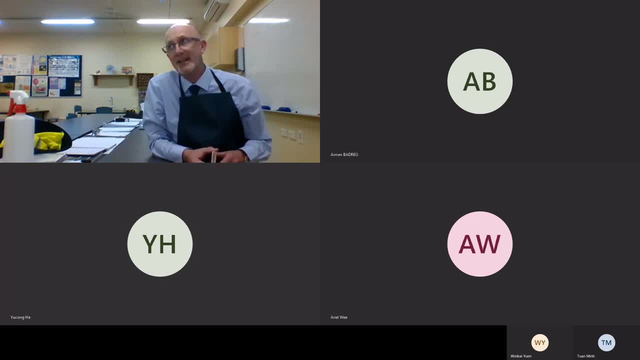 20%, 20%. okay, so it's not a lot. what's the most gas? okay, so it's not a lot. what's the most gas? okay, so it's not a lot. what's the most gas in the room that we breathe or outside, in the room that we breathe or outside? 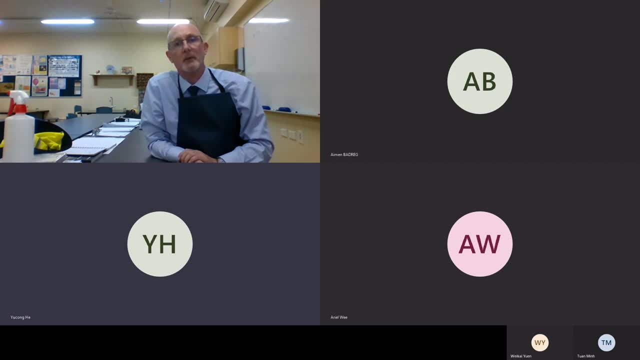 in the room that we breathe or outside? what's that gas pool? what's that gas pool? what's that gas pool? and two, which is what's the name, that's. and two, which is what's the name, that's, and two, which is what's the name. that's the formula. 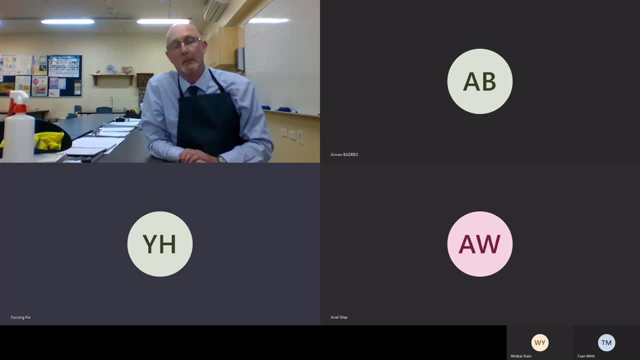 the formula. the formula: uh, let me check the p table. uh, let me check the p table. uh, let me check the p table. yep, is it, is it, is it? uh? nitrogen, yeah, nitrogen, okay, that's good. so i'm holding this magnesium ribbon with a pair of tongs because 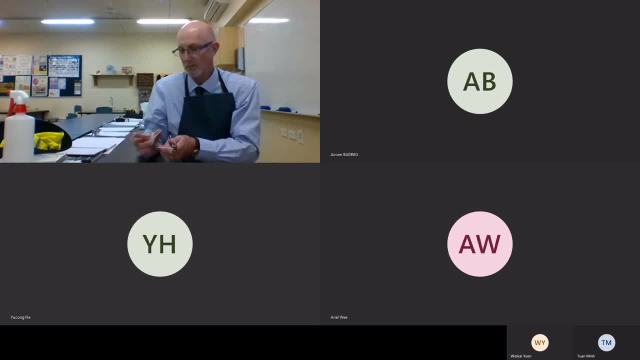 i'm going to burn, i'm going to cause a chemical reaction called combustion. okay, so this is going to burn very, very brightly. so i don't know if i'm going to destroy the camera or not, but please don't stare at it. have a glance sideways. if it's very bright, okay, don't stare at it. 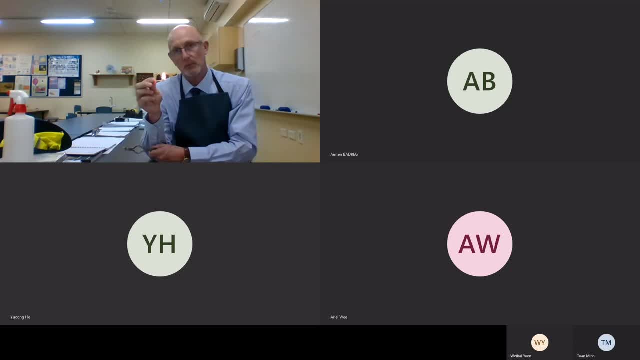 so oxygen in the air. that's a chemical reaction happening right now. okay, the carbon and the wood oxygen are burning, now oxygen and magnesium. if i get that chemical reaction going, that didn't next one, oh, one more. maybe the flame is not hard enough, i might have to get my bunsen going. 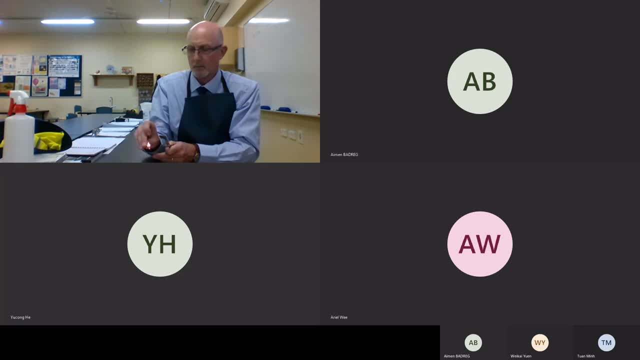 oh, nearly nearly win one more time. sir, i think you'll need the alcohol burner. yeah, i think i might. there's a bit of carbon that's carboning up because we get an incomplete combustion happening and we have a lot of carbon being produced. come on, you can do. 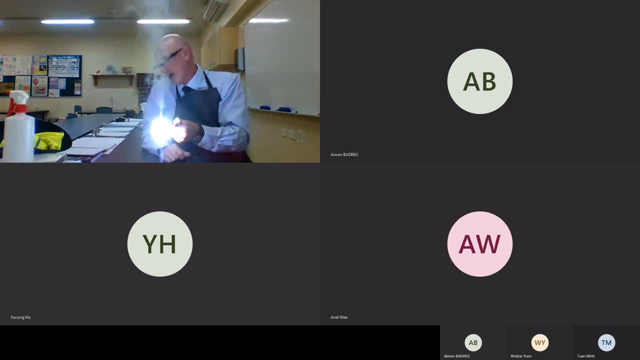 it. oh, there we go up. Okay, so that chemical reaction now is producing a lot of light. That's a sign of a chemical reaction. We get a new product. What we see there is now a white powder, which I don't want to touch because it could be hot. So now, instead of silver, it's a white. 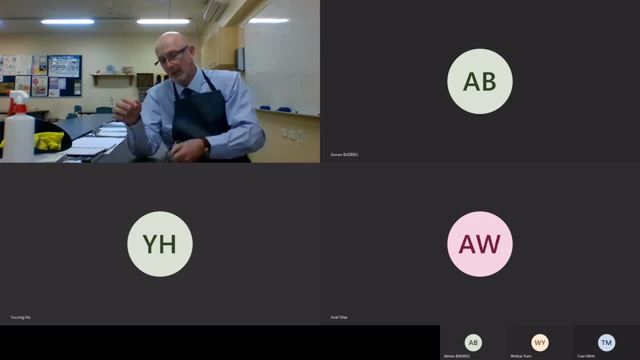 powder. It's brittle. If I touch it it'll break. So that's another sign of a chemical reaction. So the first reaction we had: we got colour change And you might be able to see some of the sediment forming down the bottom. Second reaction: we had magnesium. 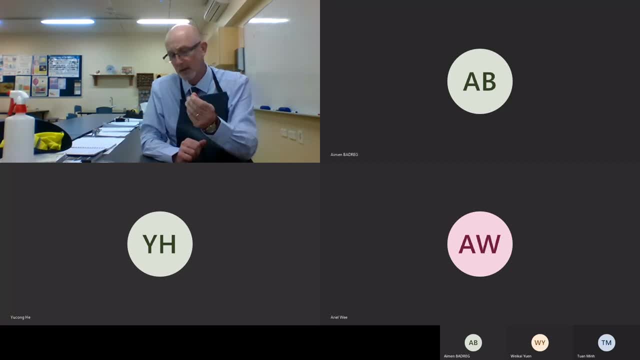 metal reacted with air, the oxygen in the air, and it produces a new product, A white powder. Now we're going to go to a third reaction, And that is this one. Okay, we have a beaker, We have hydrochloric acid. Does anyone know the formula for hydrochloric? 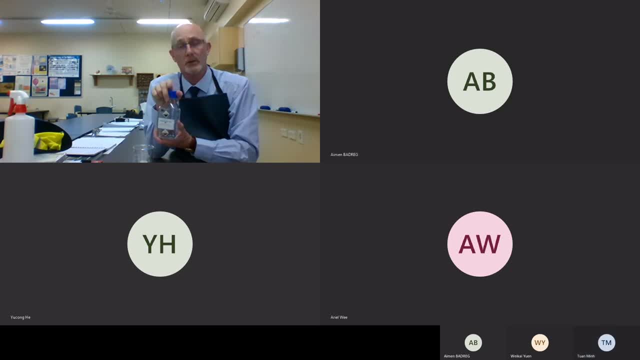 acid HCl. Very good, I was going to pick that Min HCl. So what two elements are in that Min? What two elements on the periodic table? Hydrogen and chloride, Yep, Hydrogen and chlorine. So what I'm going to do now is 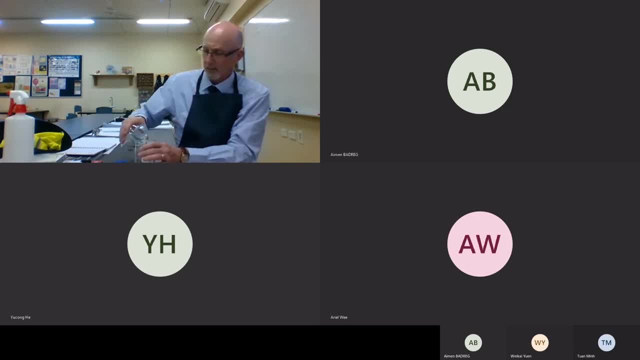 add a bucket load- Probably too much. Let me put some Back Acid. Don't want to spill that. What I'm going to do now is I'm going to take the temperature. I don't rest the thermometer on the bottom, because that means I'm taking. 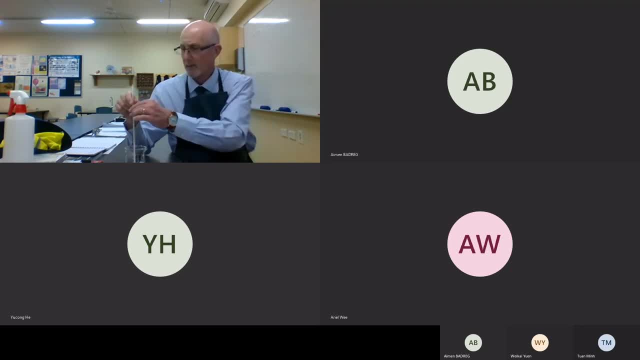 the temperature of the glass. So I have to suspend it And I should hold my thermometer near the top So my warm hands don't heat the change in temperature. because I want to take the temperature of the liquid and at the moment it's 20 degrees and it's 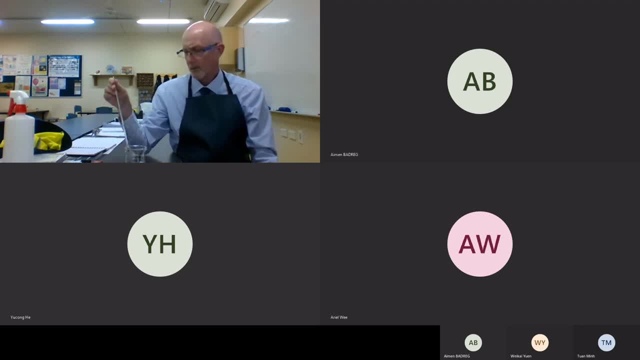 not moving. So what I'm going to do now is I'm going to put some magnesium ribbon into the acid. Can you hear that? So that's bubbling really, really furiously, Steam coming off. So now I'm putting the thermometer back in so I've got bubbles. That tells me there's 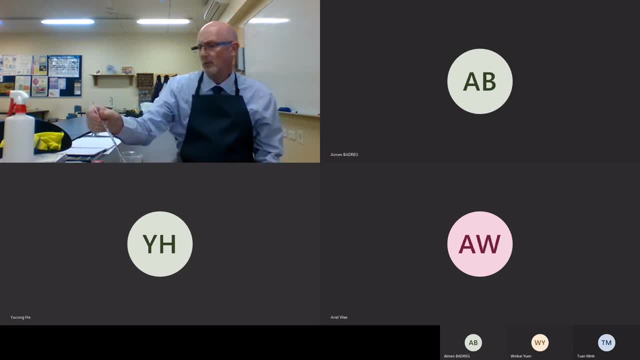 a chemical reaction Reaction happening. Now. I'm up to you, have to believe me- 23. Nearly 24.. I think it stopped just under 24.. So I went from 21 to 24.. So that's what we call an exothermic reaction. 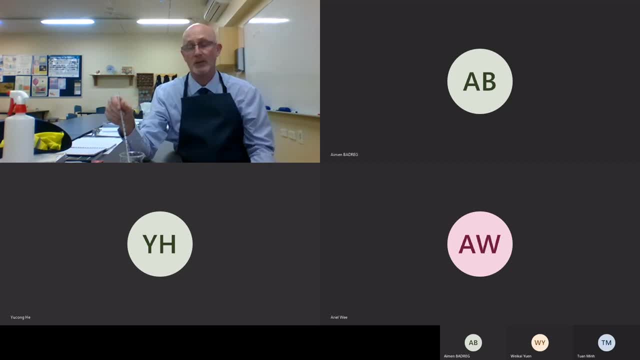 because it gave out a lot of heat, gave off lots of gas. Now if I didn't know what I gas was, that would be very dangerous because it could be poisonous. The gas it actually gave off is poisonous. I've got some. I've collected some of that gas. What I'm going 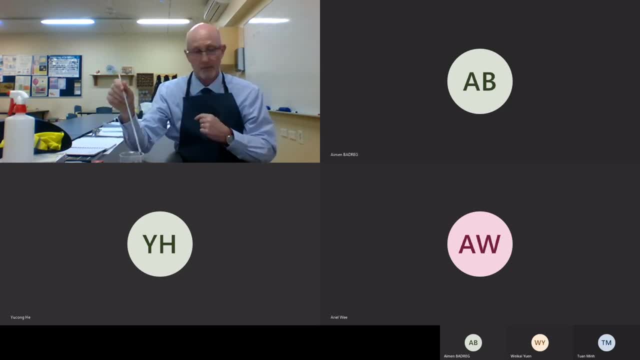 to do is I'm going to get the lab assistant that helps me with my experiments to actually bring it in and we're going to give it a flame test. We're going to see what happens when we put energy Near the gas that came off that reaction. So just stay there for a second. I'll just 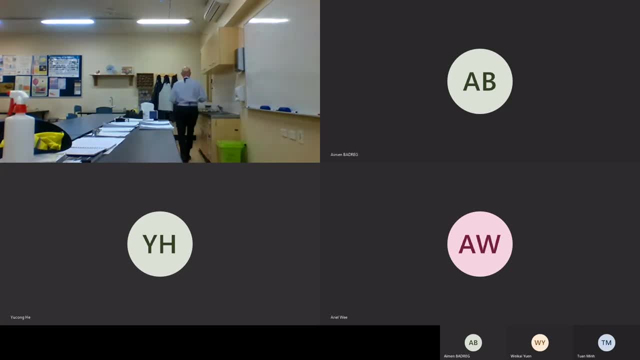 go get my assistant. Okay, wait, wait, wait, wait, wait. Now what I've got here, if I put it sideways, is a metre rule metre long, and on the end I've got a little what we call a taper, like a very small candle. 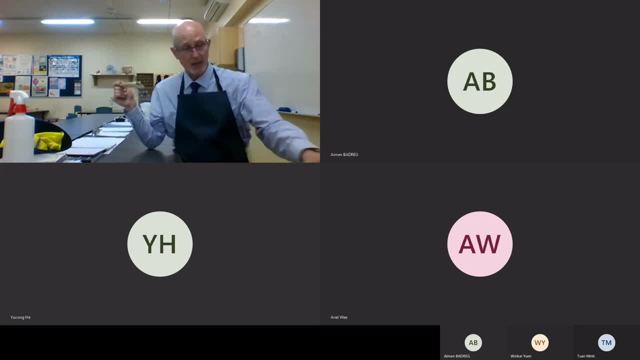 So I'm going to light this, then I'm going to see if that gas that we collected from hydrochloric acid and magnesium put it near a collection of the gas and I'll collect it in a rubber balloon. then I'll see what happens. 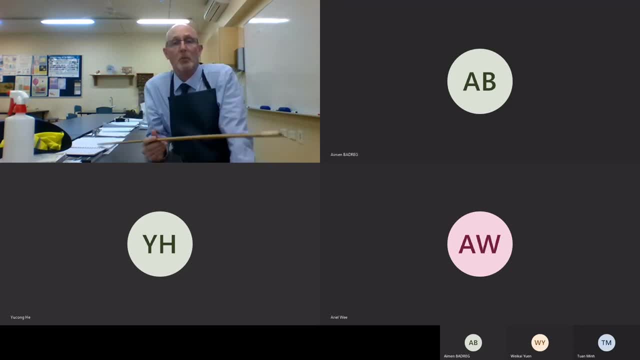 Anyone like to predict what the gas is and what would happen If you want to put it into the balloon? I think it is hydrogen And the balloon will blow. What will happen, Willem? The balloon will fly up high up to the sky. 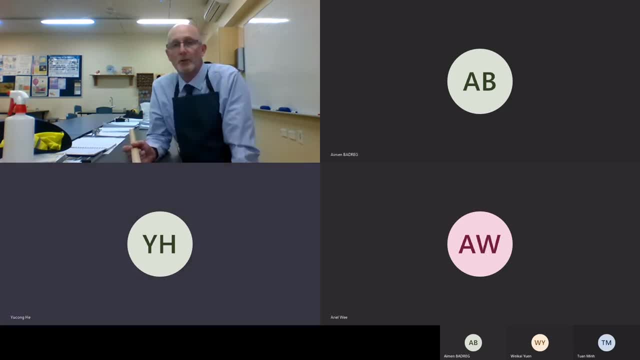 Yes, it could fly up. So do you know what the name of the gas is? Hydrogen, Hydrogen gas, Okay, So like magnesium ribbon, if we introduce a bit of energy with a flame, it might react with the oxygen in the air. 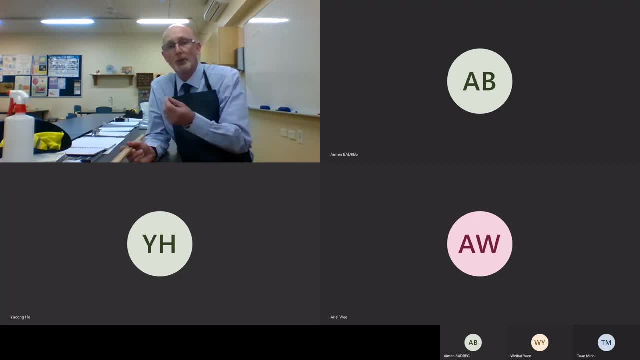 So H2, hydrogen gas Plus O2 in the air, with a bit of energy, it will make them react together and it will produce a product, or two products possibly, and we'll see what happens. okay, So that's what we're going to be doing very, very shortly, okay. 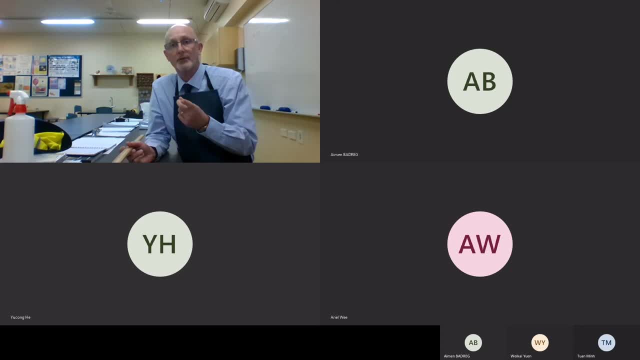 So where did the hydrogen come from? So Willem's told us it's hydrogen gas. So, Ricky, which? Where did the hydrogen come from? Okay, Where did the hydrogen come from? Did it come from the magnesium, or did it come from the acid? 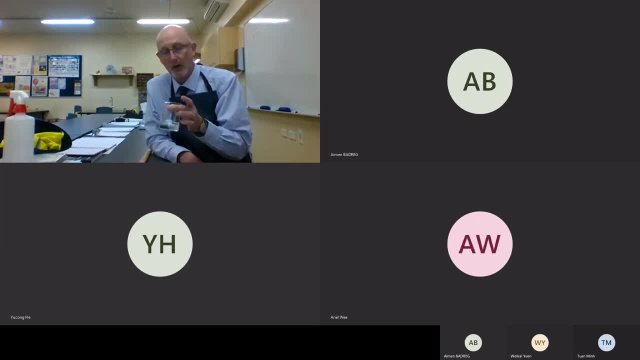 From the acid, Right? Okay, So hydrogen did come from the acid, because we know it's got hydrogen and chlorine in it. So where did the chlorine go? Anyone like to suggest where the chlorine has gone From the HCl Right? 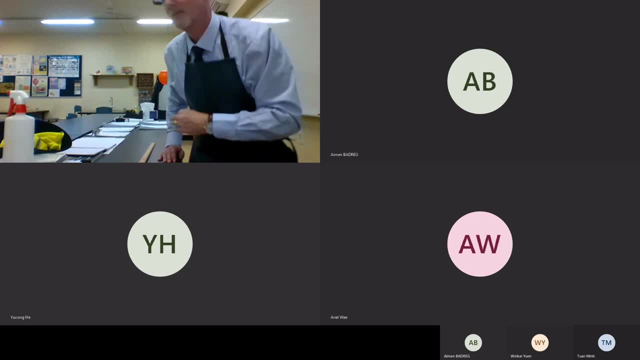 Okay, Okay, Here we have it. Can you see that balloon in the background? Let me move it a bit closer, All right, let's. Can you see the balloon? Yes, good, Let me just angle this up a little bit more. 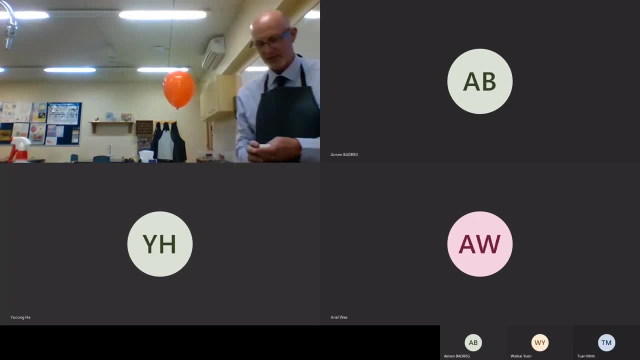 Right now you're going to have to block your ears. I'm going to try and do that For protection. I actually should have air masks. So what I will do, I will improvise. That's what we do in science: We improvise. 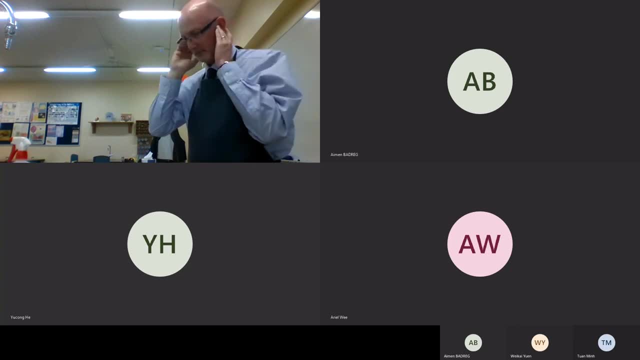 Right, That's a bit better, Right. so Willem is correct. I've tied this down. It floats. So hydrogen is very light gas, Very light. Now we're looking at the reaction of hydrogen To oxygen. Well, 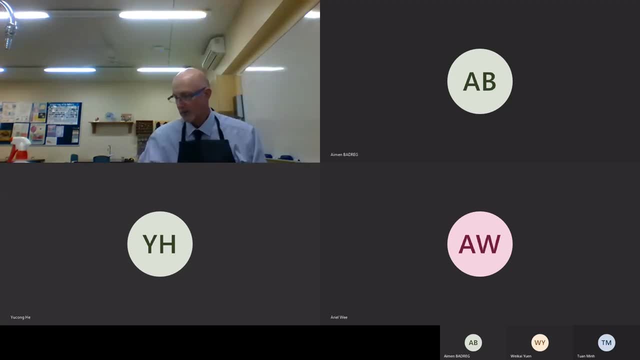 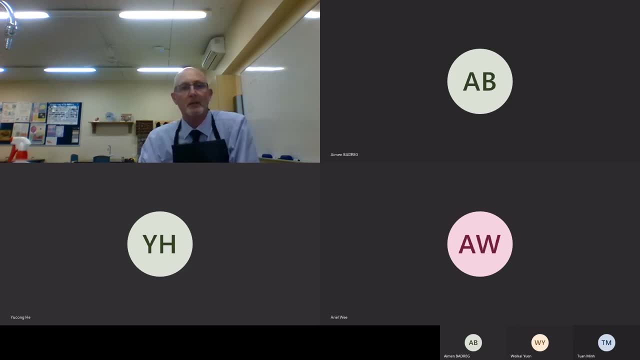 Yes, Yes, Yes, Yes, Yes, Yes. Let's make some observations. So, Eamonn, what did you see when the balloon exploded? Fire, Fire. Okay, So there was a lot of light. fire, Ricky, what else did you see? 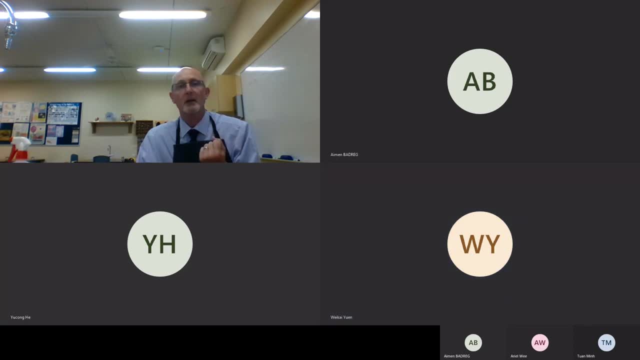 Light and fire. Okay, light and fire now. um then, if you were standing where i was standing, what would you have felt? do you think? i think you feel heat and a little sound wave. yes, that's correct. so you'd feel the heat, called radiant energy, from the ball of fire, and you would feel a shock wave. what causes the? 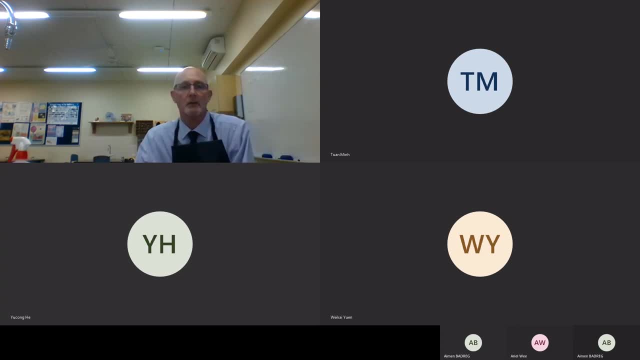 shock wave, willem? what, sorry, min, you're going to answer. then tell me: uh, the big explosion sounds, yes. what causes sound? what causes the big bang? why do we hear it? transfer of energy. it is a transfer of energy. so what happens? happens is all the gas. the hydrogen gas mixes very quickly with the oxygen. 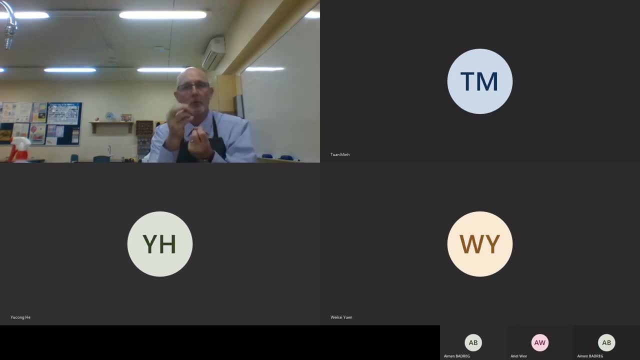 as soon as that rubber balloon goes. then you've got all this hydrogen gas, all this oxygen mixing, a little bit of energy still, and then there's a big chemical reaction and there's a lot of gas expanding and that's the bang. you hear that expanding gas, right? so that's the end of all the. 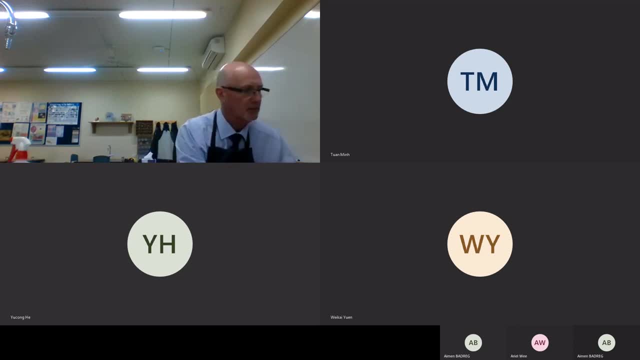 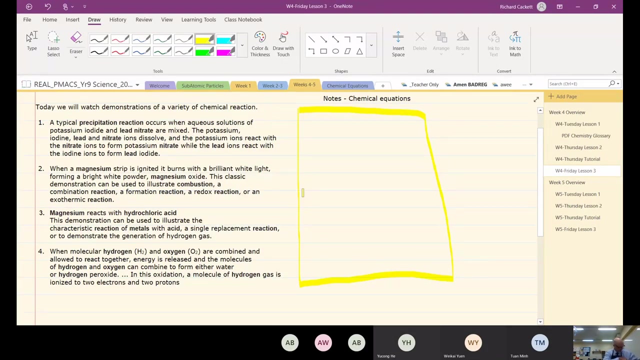 demonstrations. i'm just going to put that there and we can now start to look at our class one note, and so i'm going to share my screen now, okay, so class one note on your copies, please, not mine on your copies, please. this is where we want to document what we just did. 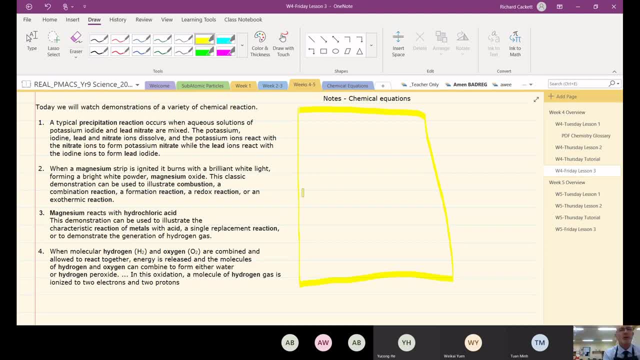 okay, so once it documented. so precipitation, okay, so lead. let's do a word word equation. so we've got lead nitrate plus vitamin E, potassium. potassium iodide. iodide gives something, doesn't it? and it says what it gives here. and so what happens? and so what happens? 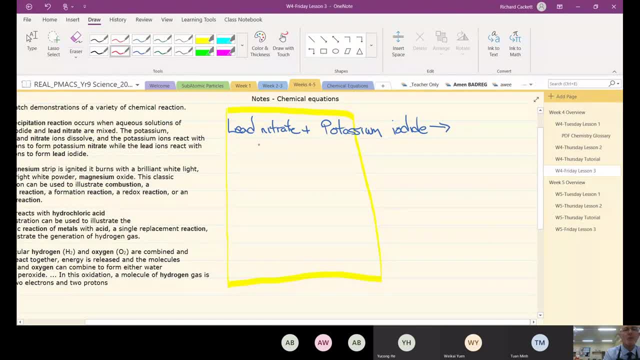 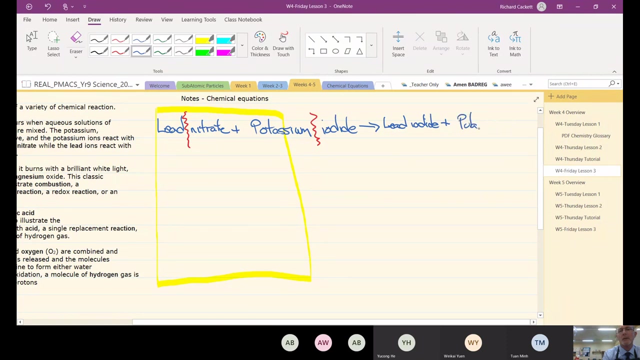 is, is they kind of swap. okay, what we get now is we get lead iodide plus potassium nitrate, and so they just kind of swap. now let's write the formulas: lead nitrate- what's the formula for lead? oh, sorry, the symbol for lead willem. 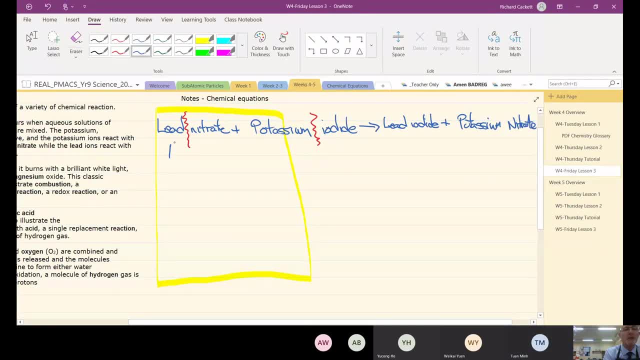 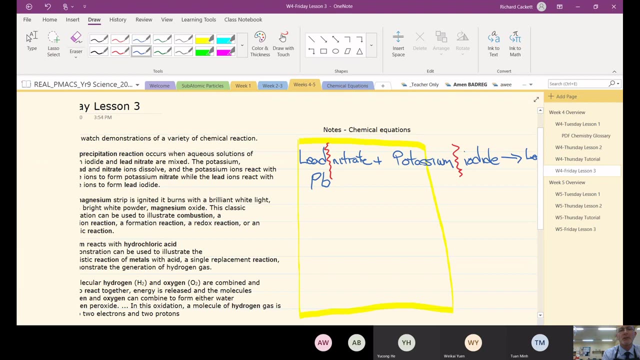 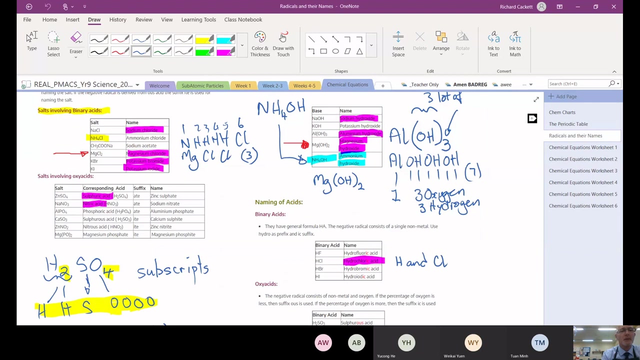 pb, pb capital, p, little b, nitrate. you know, i know the formula for nitrate. okay, this is where i'll show you where all these things are. so if i go to my chemical reactions tab and i go to radicals and names, okay, potassium iodide, i can see down there. that's just ki. 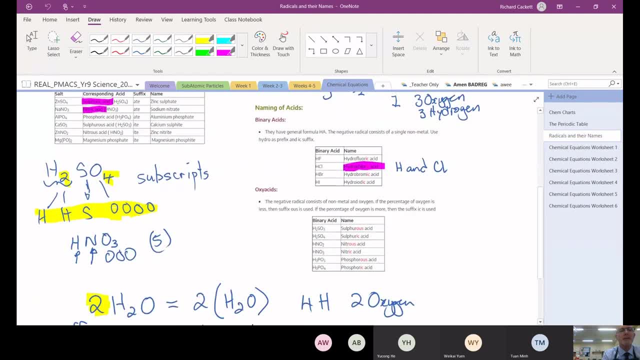 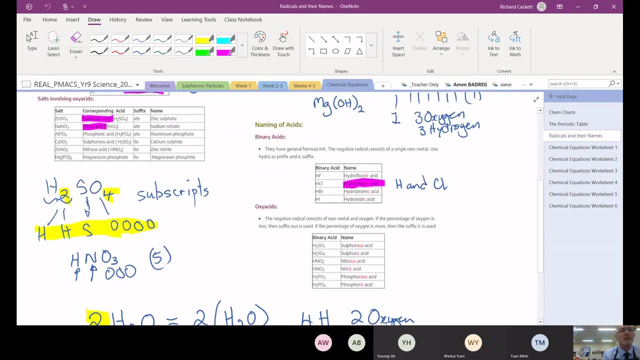 all right. so i'm looking for nitrate, something with nitrate, so i'm going to go to my chemical reactions tab and i'm going to go to radicals. so i'm going to go to radicals. so i'm going to go to radicals. okay, nitrate. 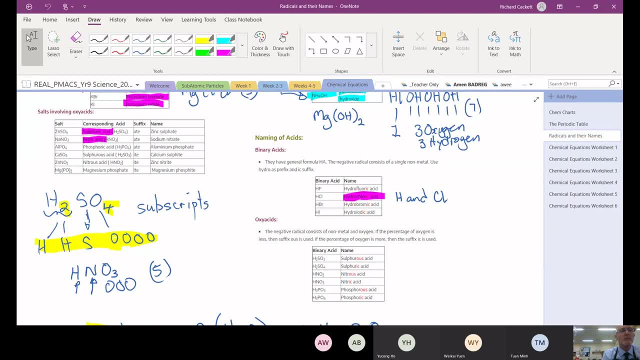 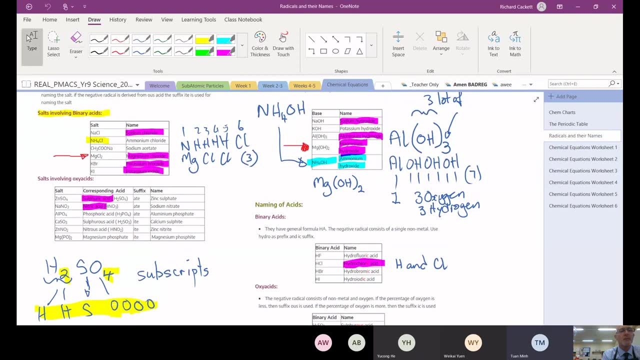 sodium nitrate. where are you reading that? uh, left the table on the left, second row. yep, sodium nitrate. so it's n? a n o three. so what's the formula for nitrate? just by itself, n o three, right? so we're looking over here for the rest of you. so it's n? o three. 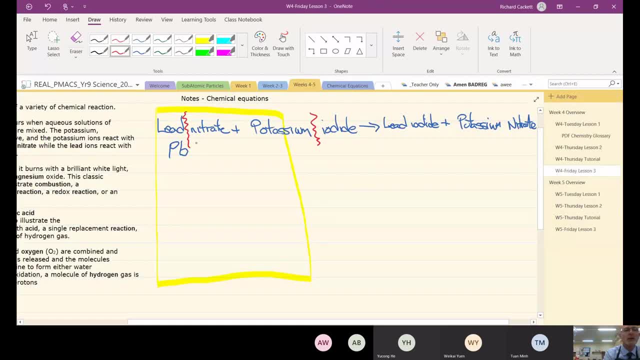 so let me go back to today's. so nitrate is n o three. now, n o three is a radical, so what we need to do is we won't worry about that. potassium symbol: k: iodine i. so k i now potassium nitrate. let me quickly just check something. 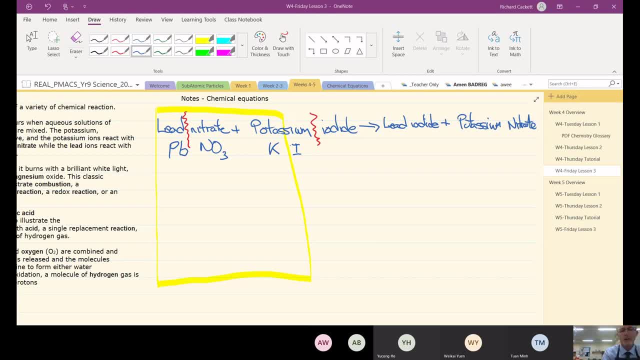 um, sorry, lead nitrate. that's what i want, so i'm just checking something: lead to nitrate, okay, thought so. now back to here. the formula for that is actually this one, okay. so the formula for that is actually this one, okay. contacting wenfosteride. so 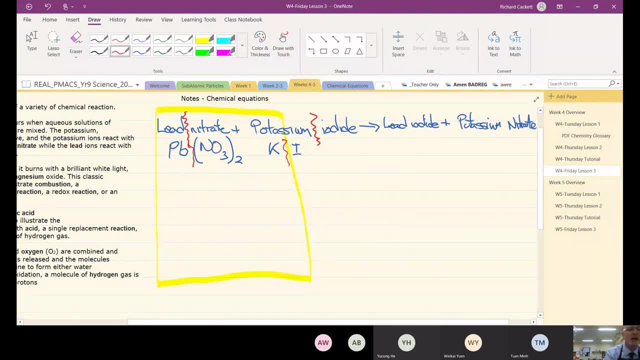 these break up, that breaks up. so now we've got lead iodide. now, before we start this pb here: lead we put in brackets two, that's lead 2.. So lead 2. That means it's got two positive charges. So if I clean up, 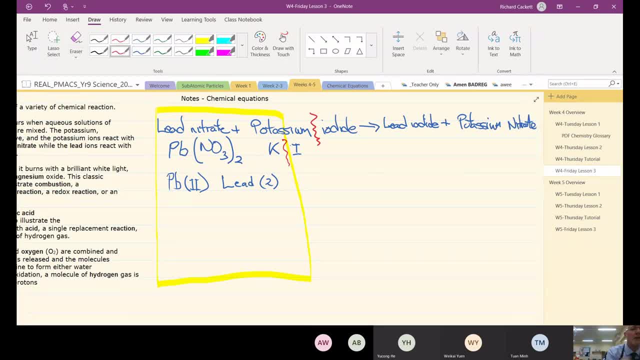 this little jagged edge. then I've got two positive charges, NO3, that's got a negative charge And I've got two of those. So the positives and negatives balance each other out. We'll do more of this next week, so don't worry if you don't understand Potassium. 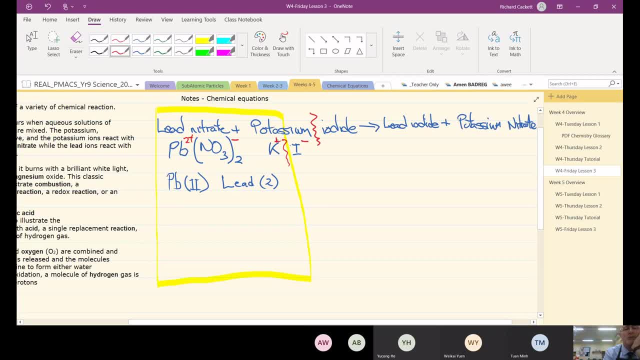 positive, Iodine negative. So one positive, one negative. cancel each other out. So now lead. So now we've got PB. It's got two positive charges, Now iodine, which is I, And it only has one negative charge. So, Min, how many iodine ions do you think we need? 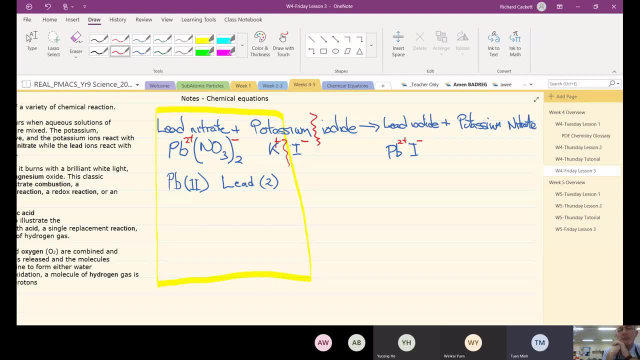 for one lead ion Two. Where would I write that two? At the bottom of I. That is correct. So you'd put it down here: So PBI2.. And you get Zero Plus that Plus. potassium symbol K Nitrate is NO3.. Potassium's only got one positive. 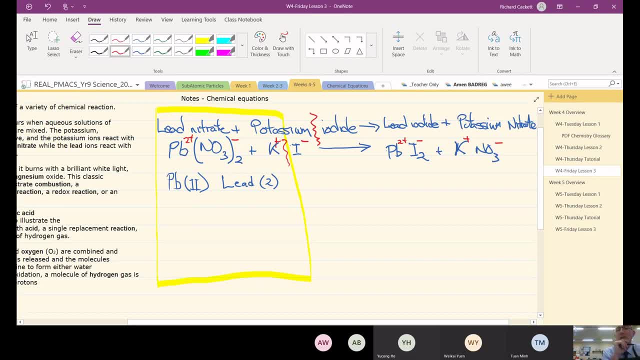 charge Nitrate NO3,. that all has one negative charge. So they cancel each other out- positive and negative- So we don't need to put any more numbers anywhere else. So that's our balanced equation for our first reaction. Okay. 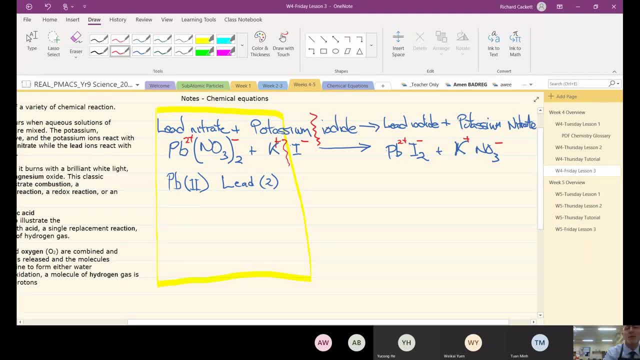 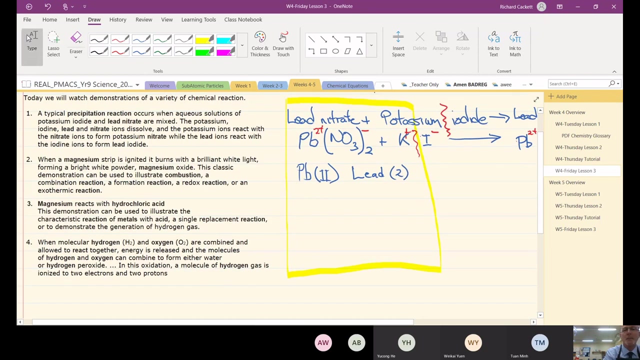 Now also, this is we put in here S for solid. Here we could put AQ because it's in solution. still Right, Amen. Let's move on to number two. Okay, Magnesium ribbon, Amen. And what's the symbol for magnesium, Mg. 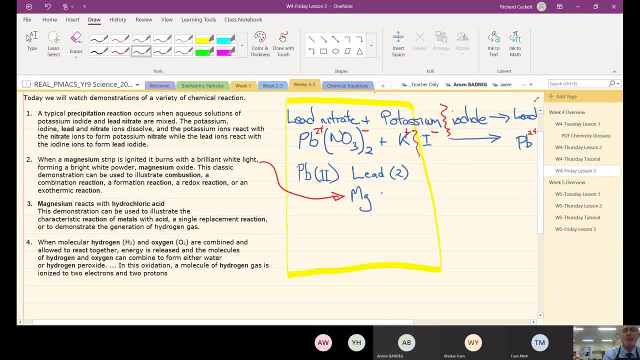 Yep, M, capital G. So there's your magnesium. What is the formula for oxygen, an oxygen molecule? Amen, O2? I'm not sure. Okay, It's O2.. So two oxygen atoms sharing electrons. So magnesium plus. 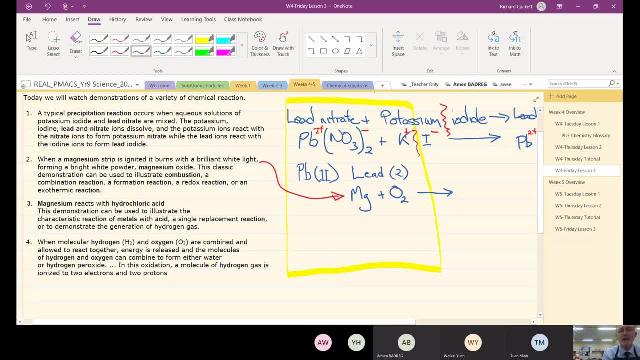 oxygen. when they react, that produces something, a white powder, MgO, Magnesium oxide. So that's a simple one. Now, is that balanced, Ricky? No, No, Where do I put the numbers? and what numbers? 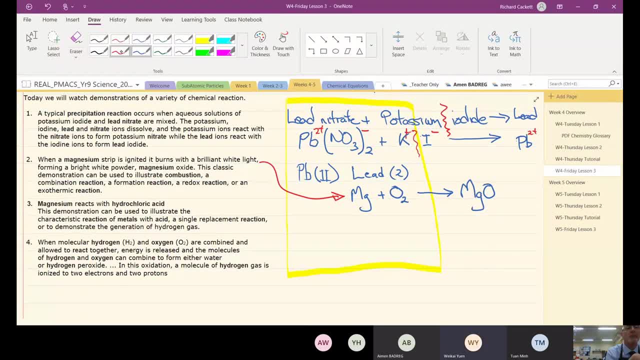 Two behind the oxygen. What do you mean? where, No, Nowhere near the oxygen. How many oxygen do I have? Two Two, Two, Two, Two. How many do I have on the left, Ricky, Two, Two. 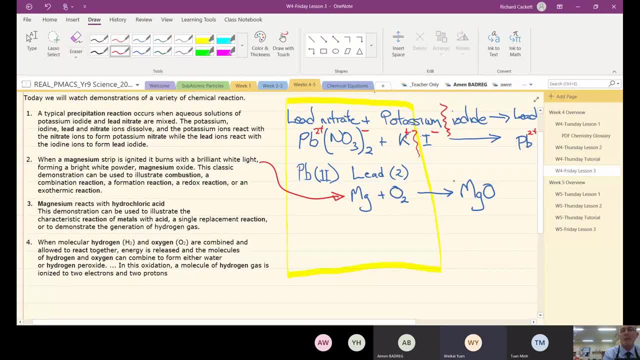 How many do I have on the right One? So that means I need to put a big two there. Now I've got two oxygen, But now I have two magnesium on the right. So how many magnesium do I have on the left, Ricky? 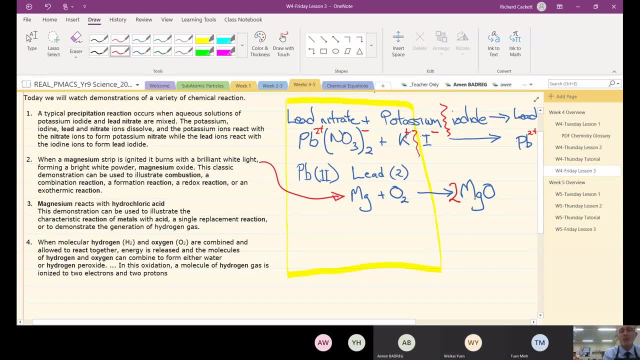 One. So I need more magnesium because I need two on the right. So I'd put a big two in front of the magnesium. I can put a one in front of the oxygen if I want. So now it's balanced Right. Number three: Willem, We know what the symbol for magnesium is: Mg Formula for: 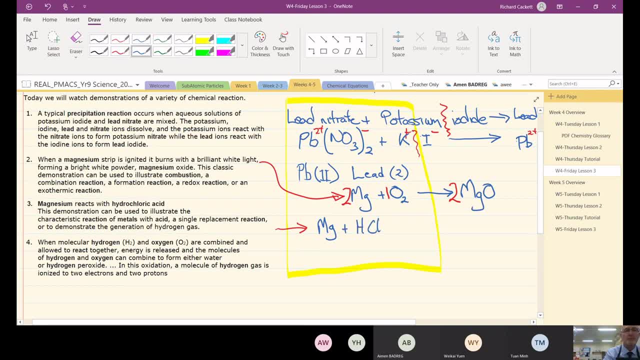 hydrochloric acid, HCl. Let me put in some charges: Mg is two plus, hydrogen is one plus and that is a negative. You correctly said we get hydrogen gas H2. Plus. what else can we make from the reactants, Willem? What other product can we make? 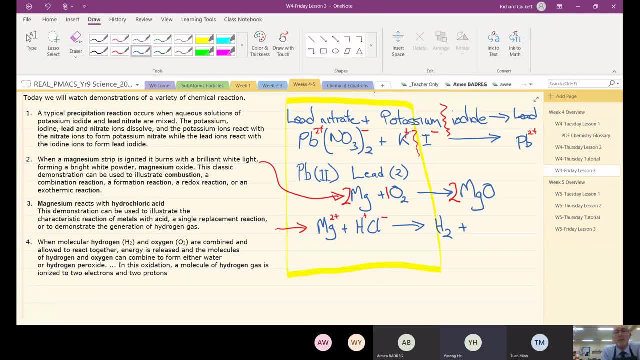 I'm not sure. Okay, Mg and Cl. Yep, So we've got an Mg and we've got a Cl. Yeah, So Mg has got two positive charges, Chlorine's only got one. So I have to write a number somewhere. Willem, Where do you think? 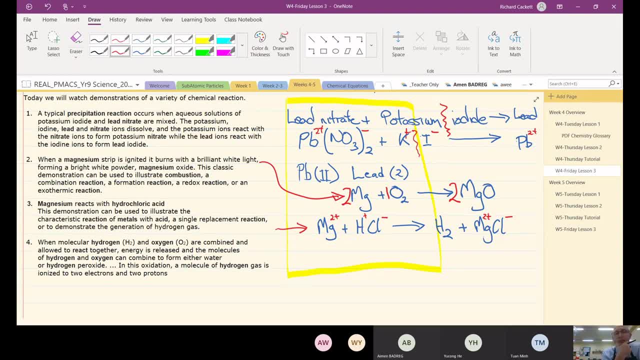 I'd write that number. and what is that number? You mean the number on the top right, No, bottom right, Bottom right. Okay, Yep, I have to write a number down here: Two, Correct. You would write the number two, because I want two chlorine to get two negative charges. 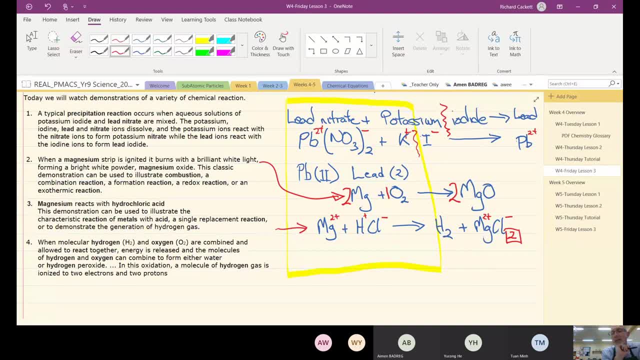 That balance out with the two positive charges for one magnesium atom or ion. Okay, Now, is that a balanced equation, Minh? Your turn now, Minh. Is that balanced? No, Okay, What do I have to do? You have to put a two before the HCl. 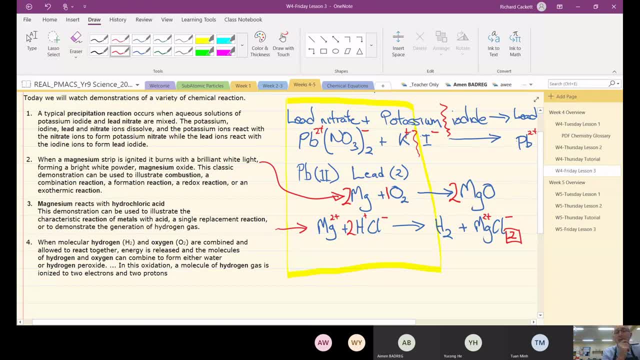 Correct. Now that is balanced. Well done Right. Last equation: Hydrogen and oxygen. And it tells you: hydrogen. We've got H2, hydrogen gas- That was in the balloon- Plus, oops, O2. Using red? still That's in the air. 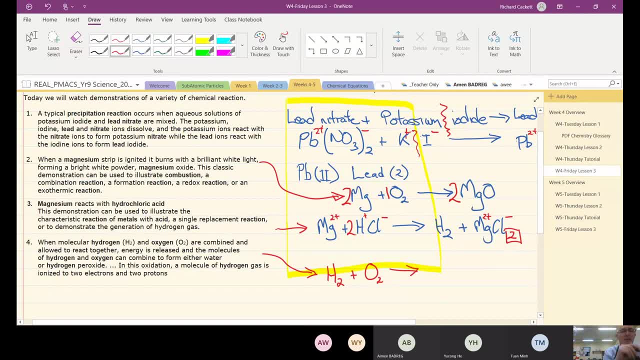 Give them a little bit of heat, Okay, And they combine to form water or hydrogen peroxide. So let's just say water, shall we? We'll just say water. So we're going to make water plus a lot of energy. 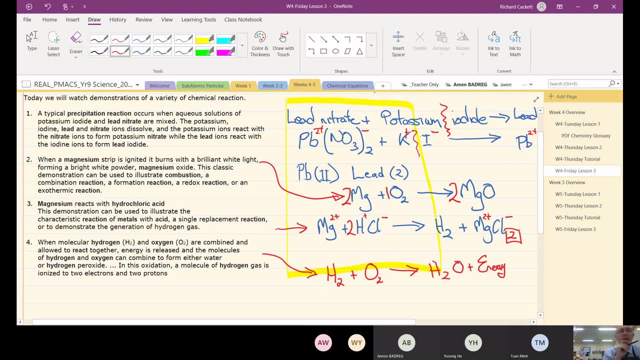 Okay, A lot of energy Now, is that balanced, Eamonn? is that balanced? Yes or no? Yes or no Eamonn, Yes or no, Yes or no Eamonn, Yes or no Eamonn. 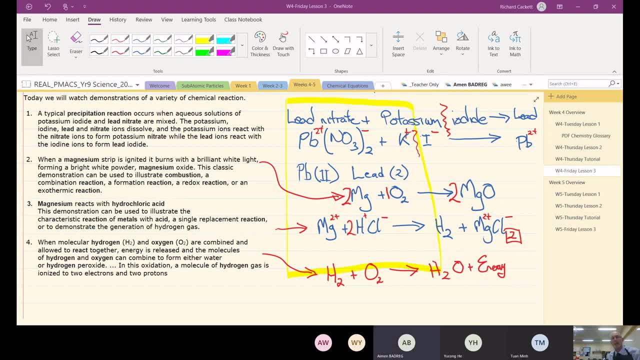 Yes, Okay, What was the question? The microphone turned off. Okay, The microphone turned off. Sorry, Can you hear me? H2 plus O2 gives H2O. Is that a balanced equation? No, there's two oxygens. 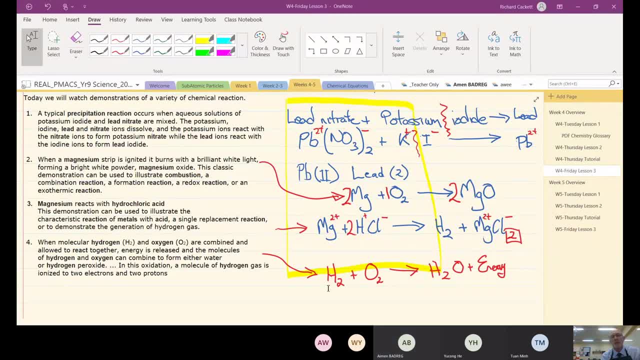 Yeah. So no, it's not Yes, And the reason why is because we have two oxygen on the left and we only have one oxygen on the right. Okay, So what I'm going to do is I'm going to leave that for homework. 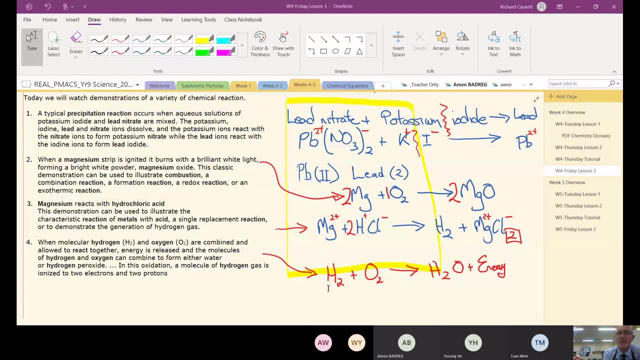 So what I'm going to do is I'm going to leave that for homework For everyone. I want you to come up with a balanced equation, please, And I will ask you that on Tuesday when we have our next science lesson. Okay, So let me just stop sharing and ask you just a couple of questions. 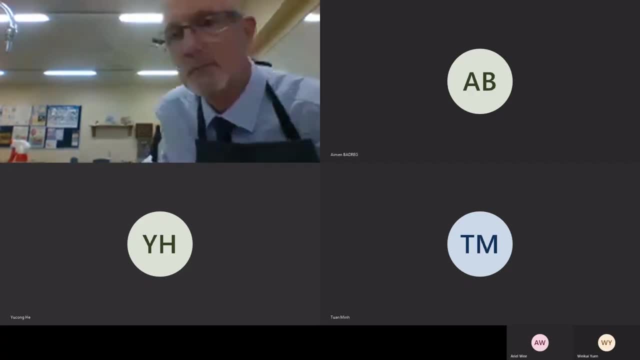 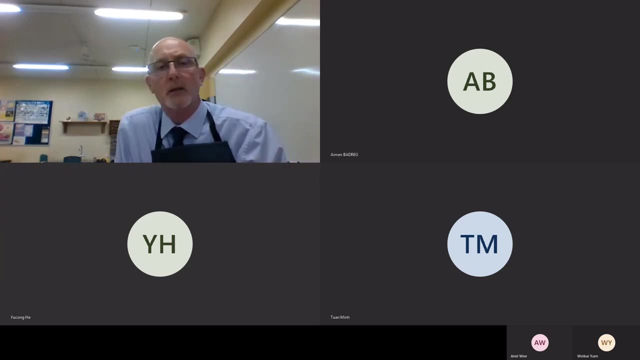 Okay, So let me just stop sharing and ask you just a couple of questions. So the question I want to ask everyone, the same question- was: this is my first demonstration of science- practicals or demonstrations. Did you find it useful? 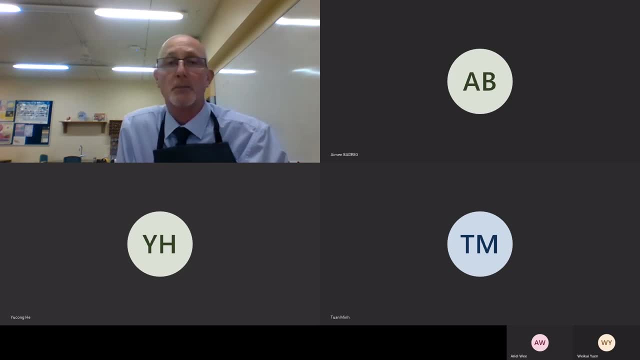 So you can give me a yes or a no And then, if you want, you can explain why you thought what you thought. So let's start in the bottom left-hand corner. So, Eamonn, did you find the demonstrations useful? 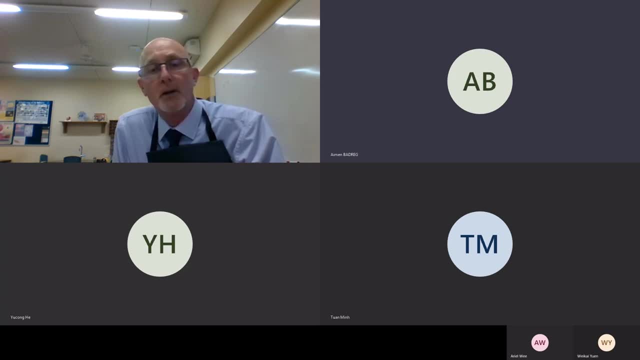 Yes, Okay, Why did you find it useful? I did not mix through liquids. I did not know that it would turn colors. I learnt with it. Okay, That's good. So, Minh, did you find this demonstration useful? Yes, 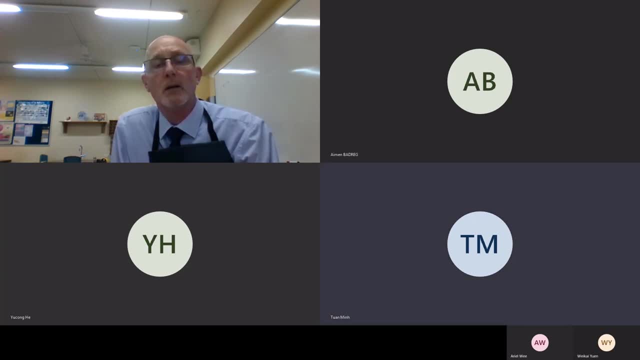 Okay, Why? I thought that your safety precautions in the class were very useful. And the last, the third experiment told me that you should never put fire in your balloon, Especially if it's got hydrogen in it. Okay, Willem, did you find it useful? 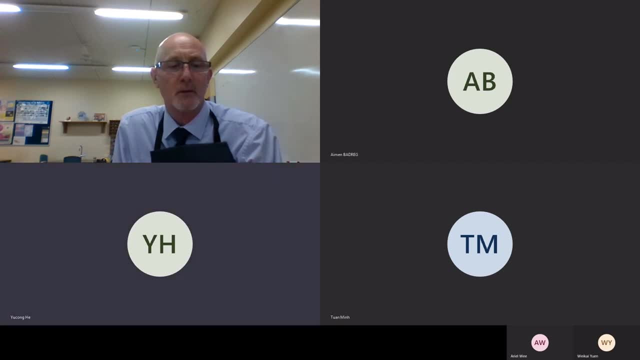 Yes, because it's easy to understand the effect of these reactions by students, not just learning it from books. Yes, I agree with you. And Ricky, what about you? Did you find it useful? Yeah, I learnt about the reactions, and watching you do it makes me feel like I'm actually next to you, and seeing you do it 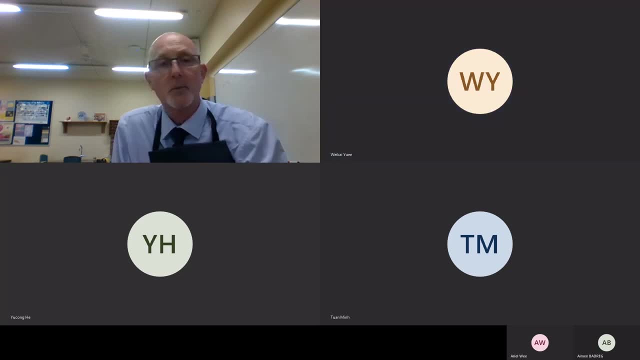 Okay, Brilliant. Now we've run over time a little bit because we've got a maths lesson, So what I'd like you to do, please, I need to move from my lab back to my office, So if I give you about three minutes, 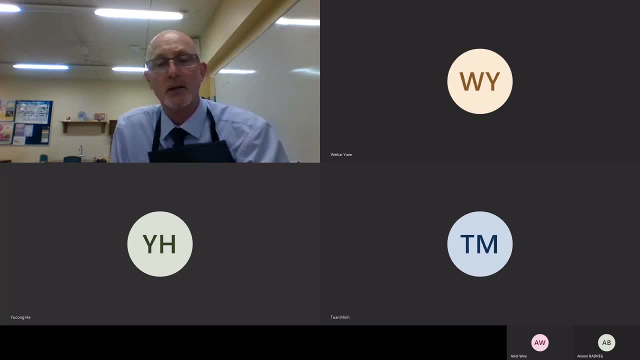 Okay For a quick drink, toilet exercise and then, if you'd like to join our maths lesson. we will finish the week off with a little bit of maths. So I'll see you everyone in about three minutes. Okay, So time to go. 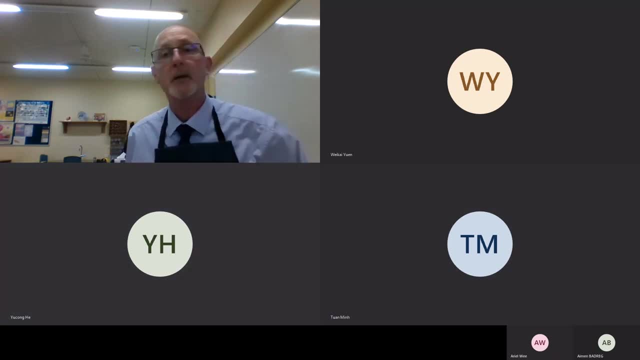 No more questions. Bye, Okay, Bye.